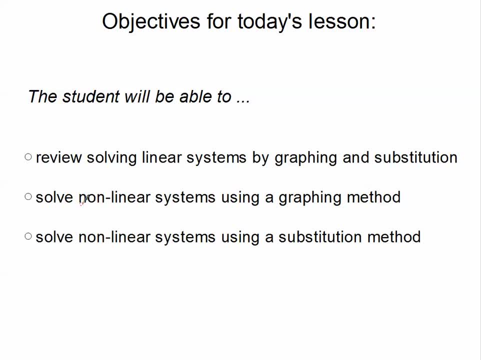 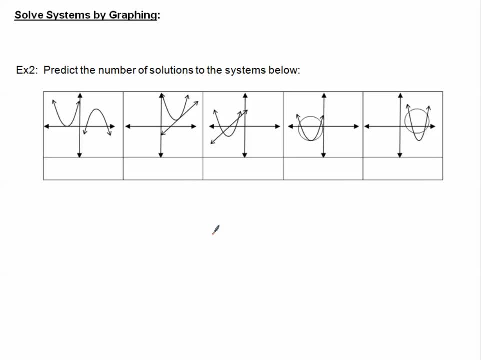 In this tutorial, we will solve non-linear systems using a graphing method. So let's flip over to example 2.. We're solving systems by graphing. Our solution, or solutions, will be where two graphs intersect. That's ultimately what we're looking for when we're looking for a solution to a system by graphing. 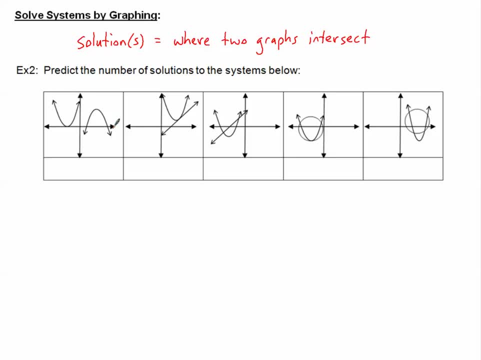 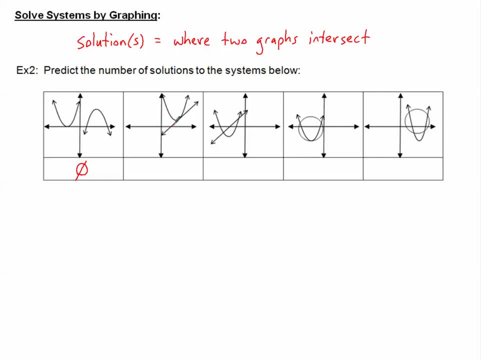 I have a parabola, it's graphed, and I also have a line, And where they are intersecting is this one spot right here We could actually use the word tangent, because this line is tangent to our parabola And there is one solution. 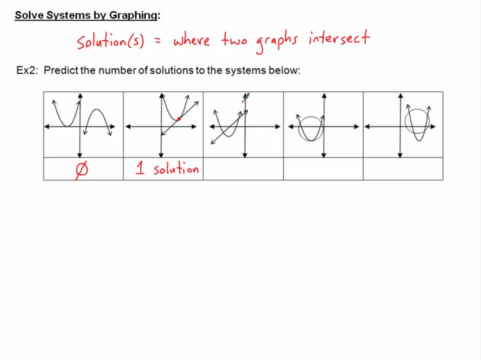 Looking at our middle case, I have a parabola and I've graphed a line. This time our line intersects our parabola in two. We could actually use the word tangent, because this line intersects our parabola in two. 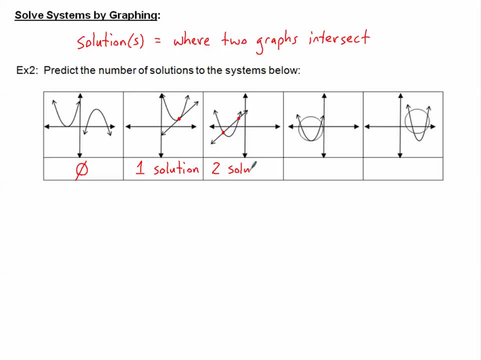 We could actually use the word tangent, because this line intersects our parabola in two. So therefore, there would be two solutions. What if we have a circle and a parabola? How could those intersect? Well, in this case it looks like we've got one solution here, one solution here and another solution right here. 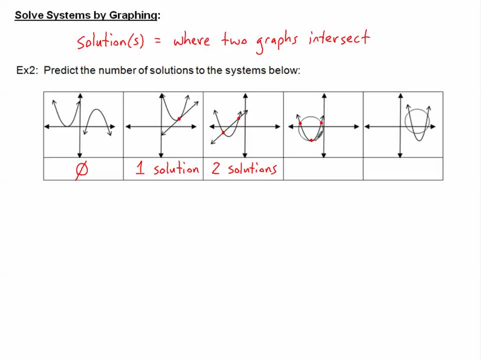 Again, it's tangent. this parabola is tangent to the inside of this circle. Three solutions and finally our last one. we have a circle and we have a parabola and this time the parabola is intersecting in four different spots. so we have four solutions. so today, when we're graphing, 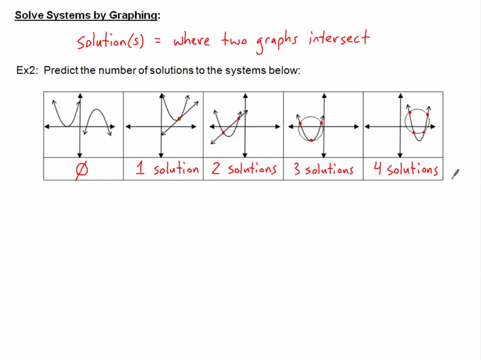 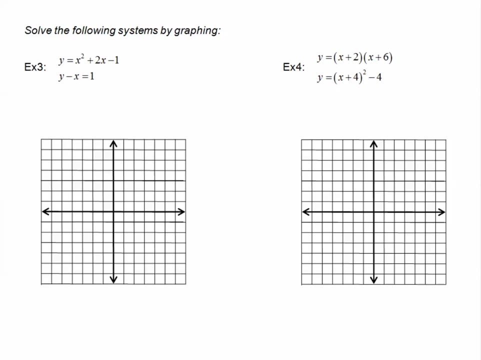 or when we're solving algebraically, there might be no solutions, but there might be all the way up to four solutions. so we're on the lookout for as many solutions as we can find. so now let's graph our own systems. i'll look at example three. i'm going to graph two equations. the first one, 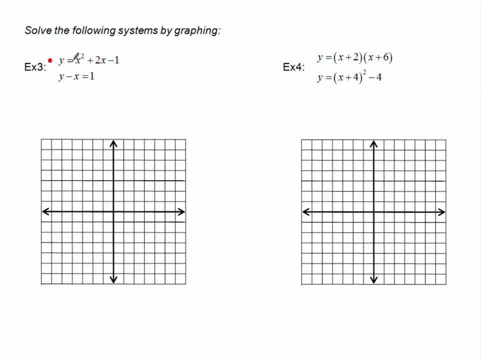 i'm just going to do in red. i'm going to color code this first equation is the equation of a parabola. it is quadratic because i see the little x squared. this quadratic is in standard form. if you you do not remember how to graph a quadratic from standard form, i suggest that you go back to that. 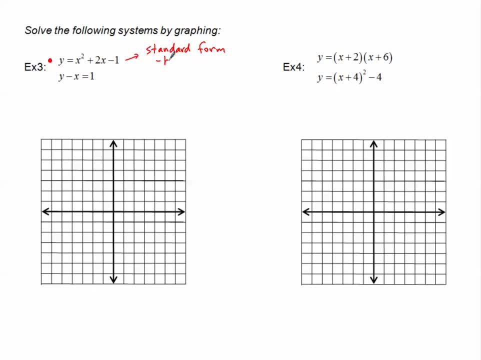 tutorial and review that standard form to find the vertex. we're going to do the opposite of b divided by 2a. so the opposite of b would be a negative 2, 2 times a. a is a 1, so 2 times that, of course, is 2, so negative 1 is what i get. that means that the vertex of this parabola is going to have: 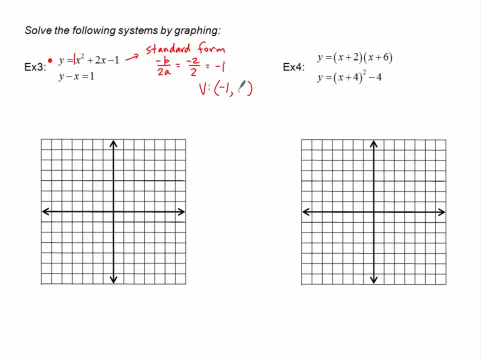 an x coordinate of negative 1. now i just need to go and find the y coordinate. once i know what x is, i can plug that into our equation to find what y is. so this is negative 1 squared plus 2 times negative 1 minus 1. so negative 1 squared is 1. 1 plus negative 2 would give me negative 1 minus 1. 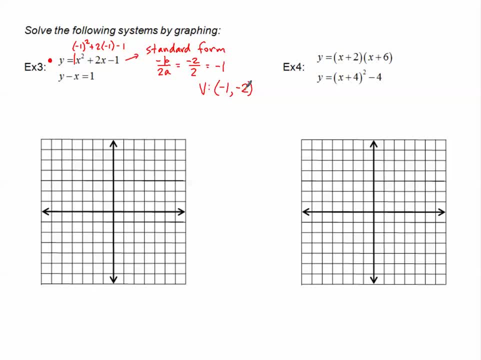 would now give me negative 2. so i have my vertex for this parabola. i'm going to go to negative 1, negative 2 and remember, i like to put a little star at my starting point. the value of the vertex is going to be negative 1 minus 1, so i'm going to go to negative 1 minus 1. 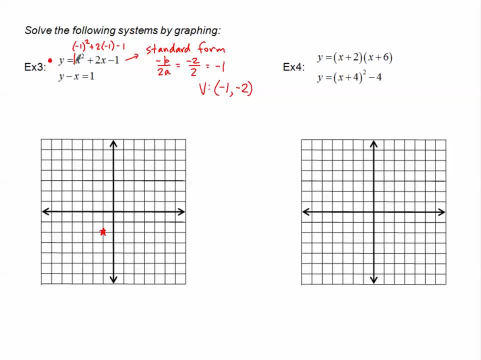 the value of a is 1 and that will help me to find all of our other values. that's our normal output. so for a parabola, when i input a 1, i output a 1. so go to the right 1 and up 1 back to the. 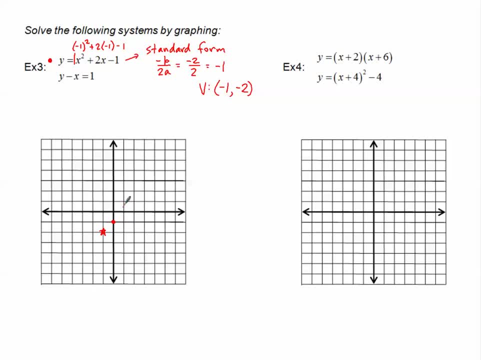 star. i'm going to input a 2 and go up 4, because 2 squared 1, 2, 3, 4. back to the star. input a, 3, 1, 2, 3. output 3 squared 1, 2, 3, 4, 5, 6, 7, 8, 9. that's probably all i'm going to fit over there. i'm going to do. 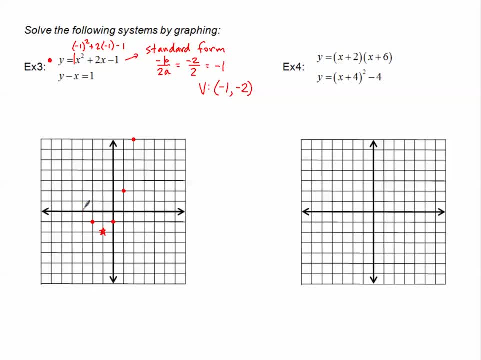 symmetry on the left side. so next we're going to do symmetry on the left side. so now we're going to negative 1, 1, negative 2, 4, and negative 3, 9.. So there's my parabola. 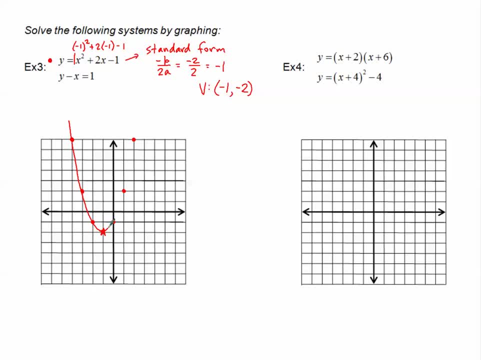 Again, if you forget how to graph from standard form, we have a tutorial for that. Go back and watch that to remind yourself. So that's our first graph. The second graph I'm going to graph in blue. This is just a graph of a line. 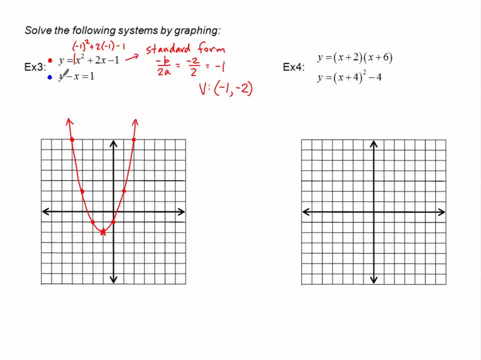 I don't see any squared terms, So this is just a line I'm going to solve for y. to put it into y equals mx plus b form, So I will add x to both sides. I will have y equals x and 1 are not the same or like terms. 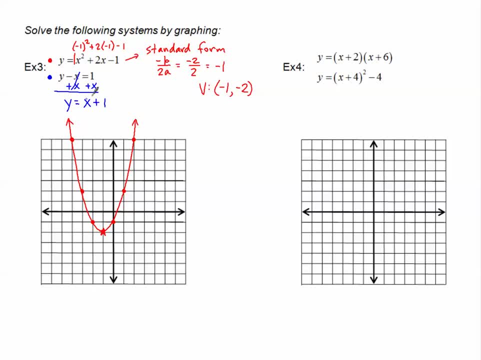 so I'll just write them side by side: x plus 1.. And now I can find my y-intercept, which is positive 1.. So I'll go to the y-axis and put a 1. And my slope is 1 over 1.. 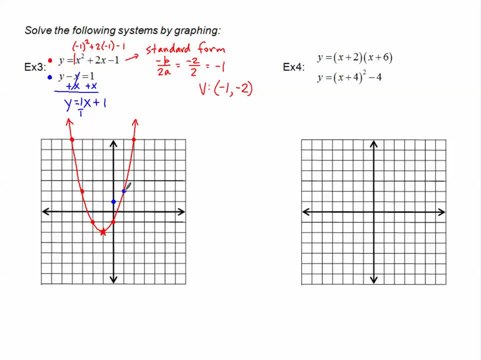 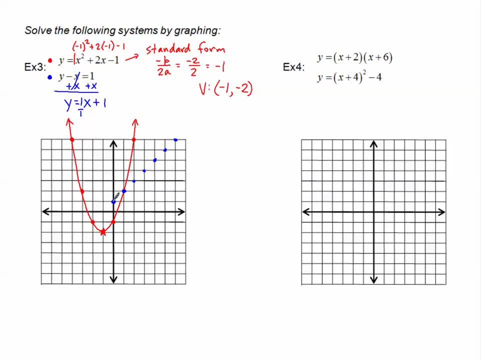 up 1 and right 1, up 1 and right 1.. And I'm going to come over here and do something like this. So I'm down and left, down and left. Hey, look at that, There's another solution. 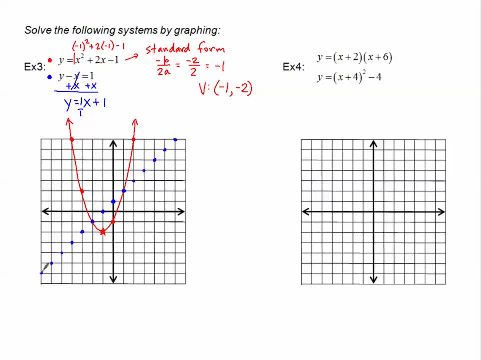 Down and left, down and left down and left. I'm going to graph as many points as possible. The more points you have, the easier it is to draw a nice straight line, unless you would like to use a ruler. So I've graphed both equations. 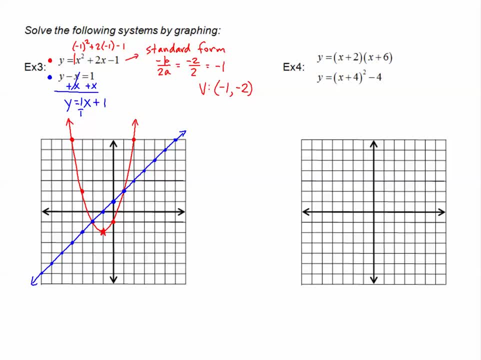 and now I'm looking for the solution to this system. The solution is where they intersect. Here's one of the solutions and here's the other solution. All I need to do is name those orderlies. I'm going to call them ordered pairs. 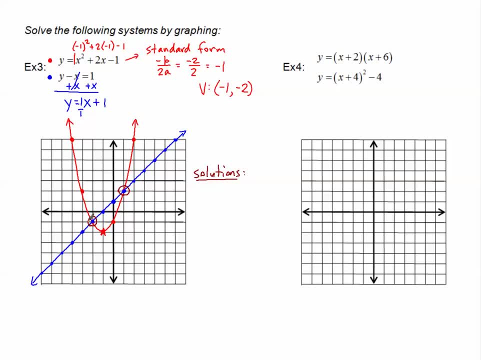 and I will be finished. My solutions are- I'll start on the left side. This is negative 2, negative 1.. That's one of our ordered pairs, And this one is positive 1, positive 2.. So we have two solutions to this system. 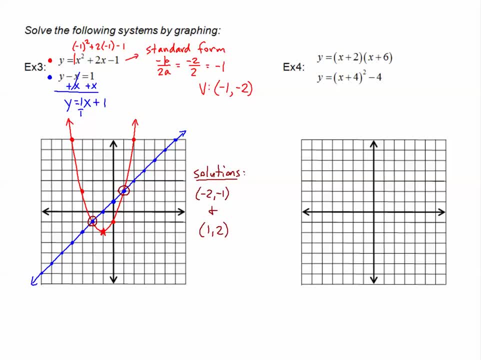 and we found them. Let's look at example 4.. I'm going to color code again. The first one I'll do in red. This is also a quadratic equation. This is also a quadratic equation. I know that because if I foiled 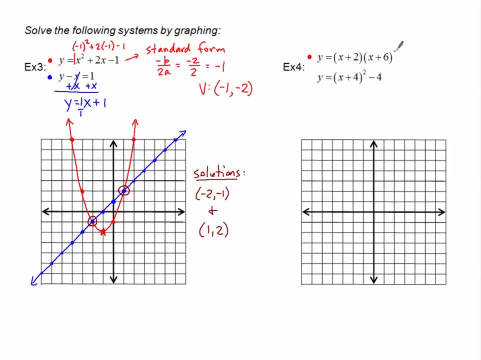 I would have an x squared, So this is quadratic. This is actually an intercept form. If you do not remember how to graph from intercept form, I suggest that you go and watch that tutorial to remind yourself. Intercept form will give us the two x-intercepts. 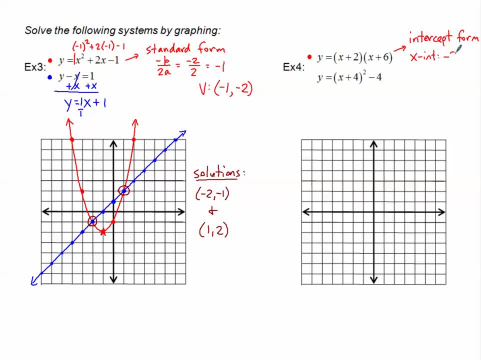 The two x-intercepts. in this case, from this factor we have a negative 2, and from this factor we have a negative 2.. So we have a negative 6.. So I know that the x-axis is going to be hit at the negative 2,. 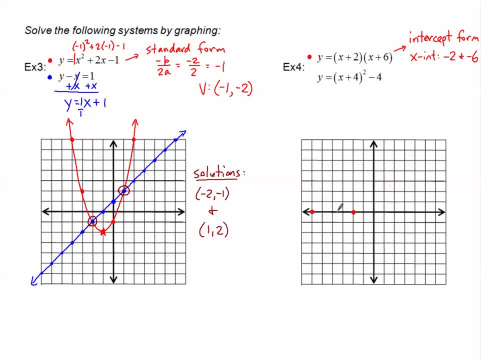 and at the negative 6.. So that's where this graph will cross the x-axis. Now I know that the vertex is going to be exactly in the middle, which will be somewhere right here, at 1,, 2,, 3,, negative 4.. 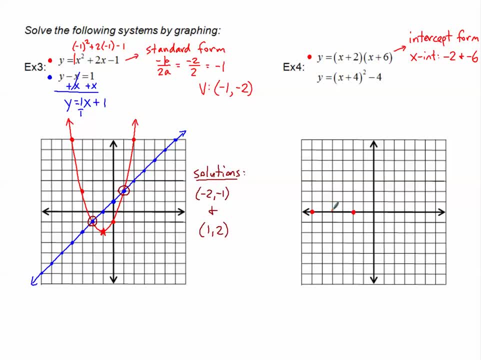 That's where our axis of symmetry would be when x is negative 4.. So I know my vertex is going to have an x-coordinate of negative 4.. I just need to find my y-coordinate So I can plug in negative 4 into our function. 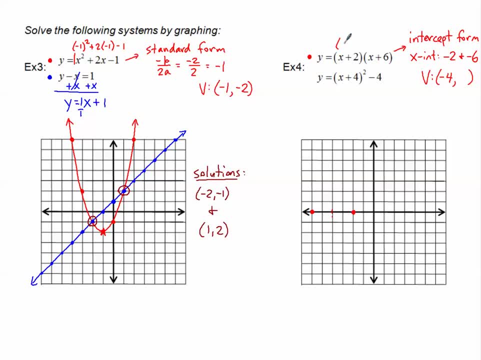 So I can plug in negative 4 into our function. So I can plug in negative 4 into our function. So negative 4 plus 2. And negative 4 plus 6. And multiply all this together: Negative 4 plus 2 is negative 2.. 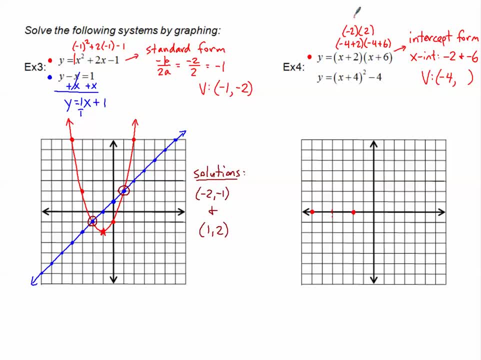 And negative: 4 plus 6 is positive, 2. And negative: 4 plus 6 is positive, 2. That gives me a negative 4. So my y must be negative 4.. So my vertex is negative 4, negative 4.. 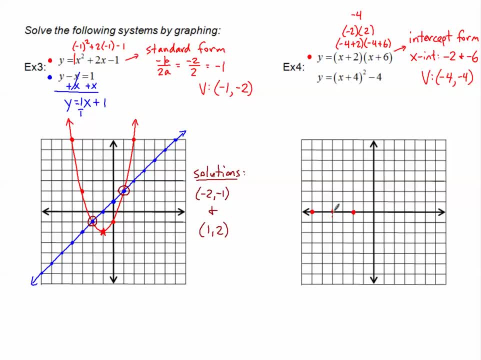 So negative 4 to the left And negative 4 down: 1,, 2,, 3, 4.. I'll put a little starting point right there And let's check my a. My a is still a 1.. 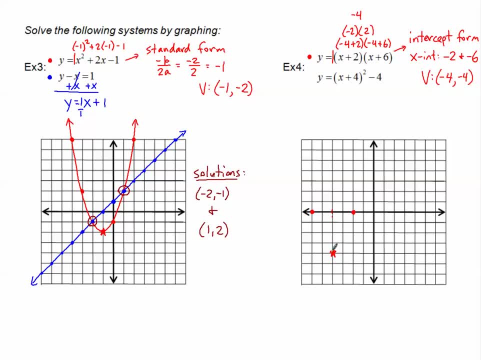 That's nice. That's my normal outputs. So from my star I'm going to go over 1 and up 1.. So from my star I'm going to go over 1 and up 1. And over 2 and up 4.. 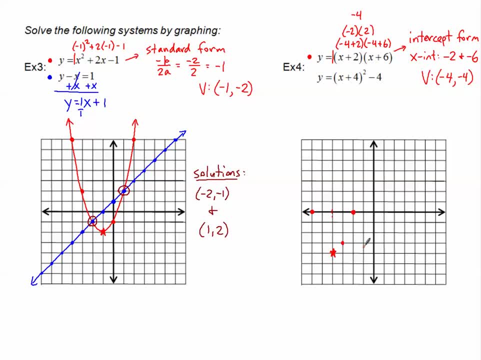 And that's a nice way to check myself, because that's correct. And one more over 3 and up 9.. 1, 2, 3, 4,, 5,, 6,, 7,, 8,, 9.. 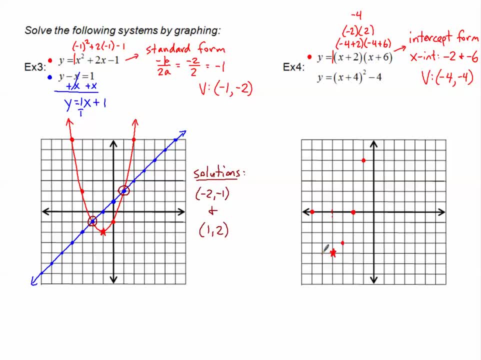 1, 2,, 3,, 4,, 5,, 6,, 7, 8, 9.. Let's do symmetry on the left side: Negative 1, up 1.. Negative 2, up 4.. 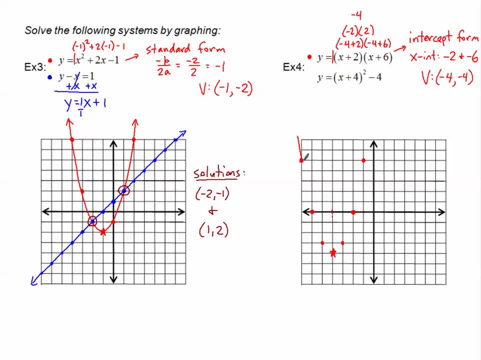 Negative 3, up 9. And we'll do a nice smooth parabola. And we'll do a nice smooth parabola. So that's our first equation. So that's our first equation. Let's graph our second equation. 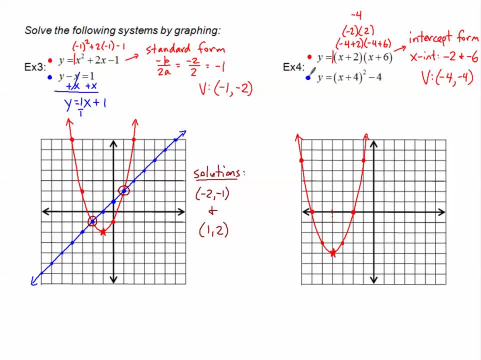 Let's graph our second equation. I'll do this one in blue. This again is also a quadratic, because I see the little x squared. This time we are in vertex form. If you do not remember how to graph from vertex form, I suggest you watch that tutorial. 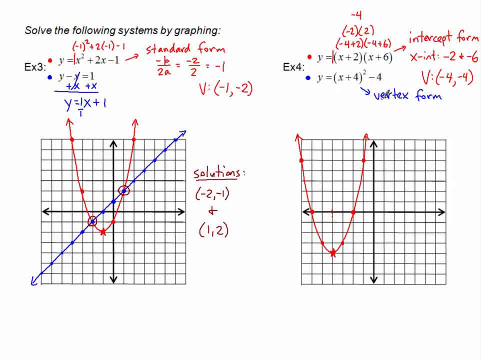 There were three ways that we learned how to graph a quadratic: Vertex form, intercept form and standard form. So this is a nice review of all three of those. Vertex form is pretty simple to find the vertex. The vertex comes from h and k. 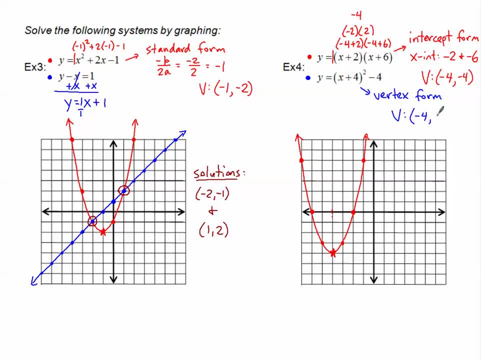 h is a negative 4, and k is a negative 4.. The easiest way to find the vertex from vertex form. So 1,, 2,, 3, negative 4.. 1, 2,, 3, negative, 4.. 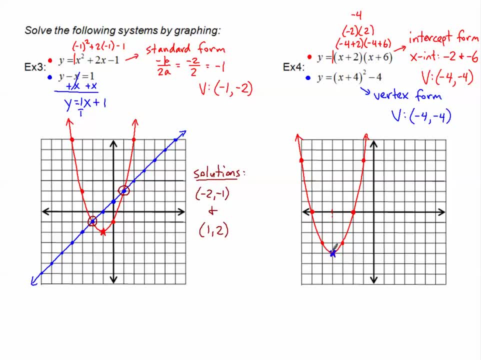 Oh, that's weird. They have the same starting point, So that must be one of the solutions, because obviously they're intersecting right here. Let's check our a. Our a is a value of 1. That's our normal output. 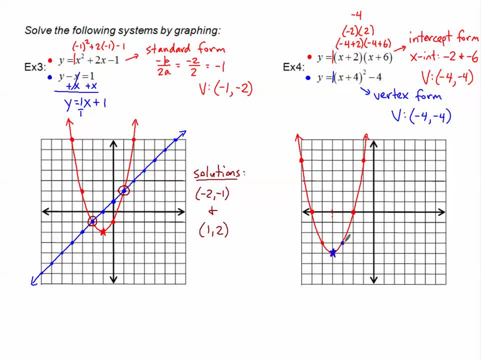 So that means from our star. when I go right 1, I go up 1.. Hey, look at that, I'm on the same parabola. When I go right 2, I should go up 4.. Huh, same thing. 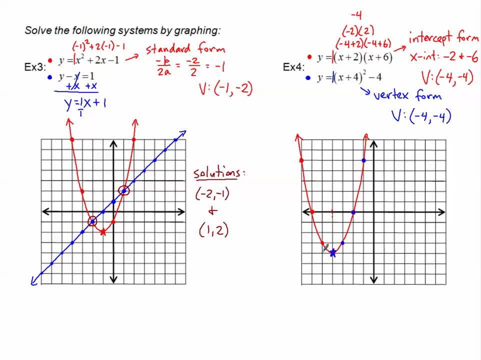 When I go over 3, I should go up 9.. When I go left 1, I go up 1.. Left 2, up 4.. Look at this: This is the same exact parabola. Every single dot that I had on that red curve. 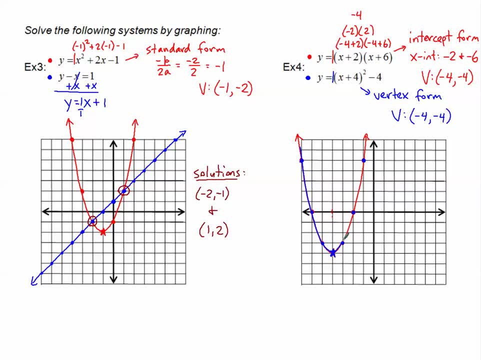 is now on our blue curve. Well, that is very interesting. If I'm looking for the intersections, they intersect everywhere, Every single point. where they touch, they touch. So what am I going to say for our solutions? I'm going to use the word infinite. 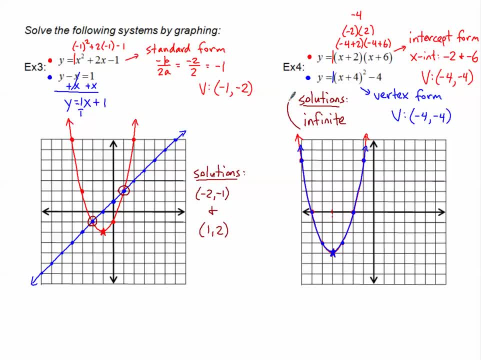 This system has infinite solutions. In fact, these equations are identical. They might be in two different forms, One's in intercept form, The other one's in vertex form, but they actually are the same exact parabola. So we have infinite solutions.